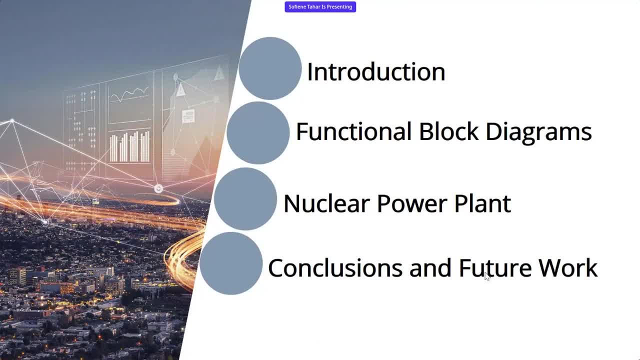 to start with an introduction. Okay, thank you. So the first thing I'm going to do is I'm going to talk about the functional block diagrams, which are the modeling, basically platform, that we use to model and analyze the safety of a nuclear. 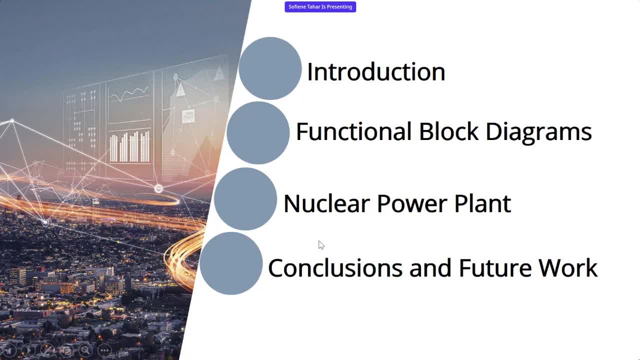 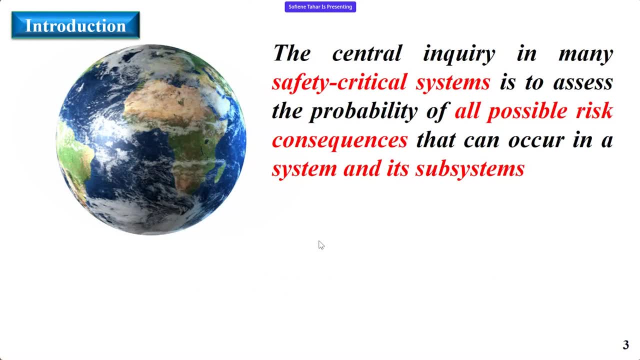 power plant. Then I conclude with some summary and some future work hints. So the central inquiry in many safety critical systems, as you know, in this workshop is really to try to assess safety of systems using formal methods, And we are in particular interested in what we call risk. 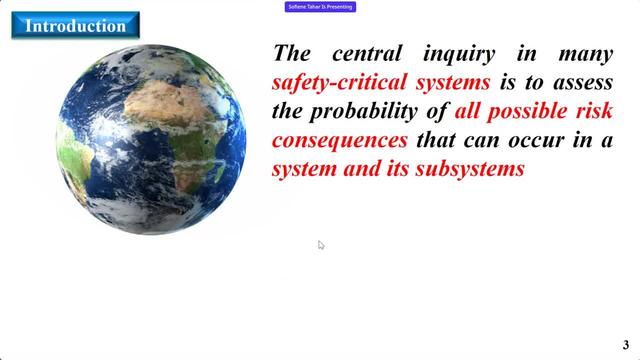 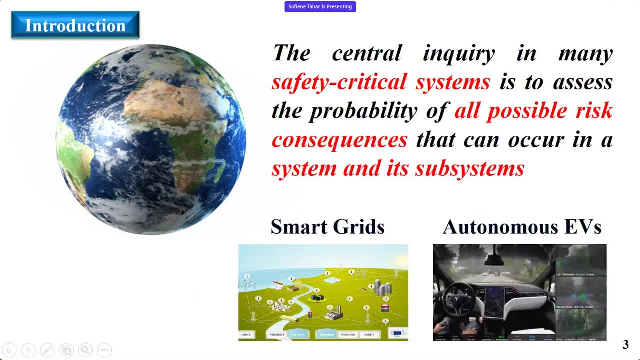 assessment that can occur at the system or at the subsystem level. So, for example, if we consider a smart grid, so it's composed of many subsystems and then so we want to consider at the same time the system as a whole, as you know subsystems, like you know parts of the grid. 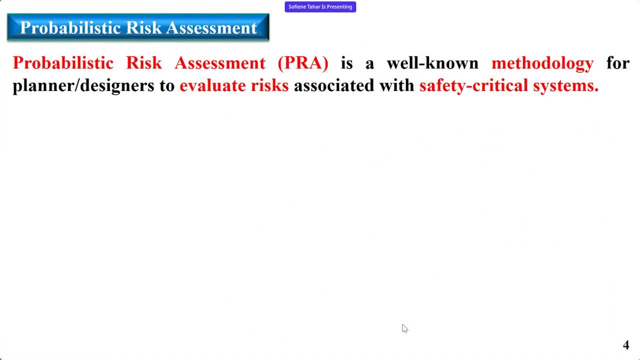 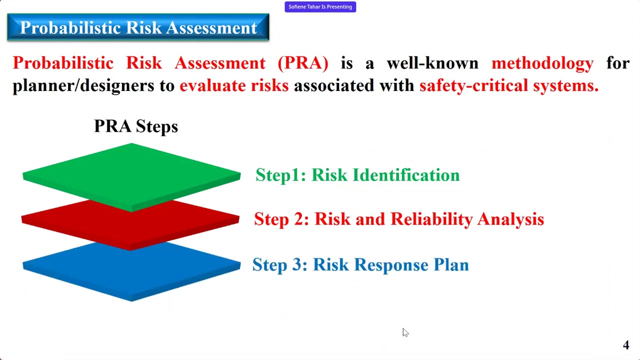 In general. probabilistic risk assessment is a known methodology for planners and designers to evaluate the risk associated with safety critical systems. They usually go through a number of steps. First of all, they need to identify the risk. Then they need to conduct a risk and reliability analysis. After that they have to come up. 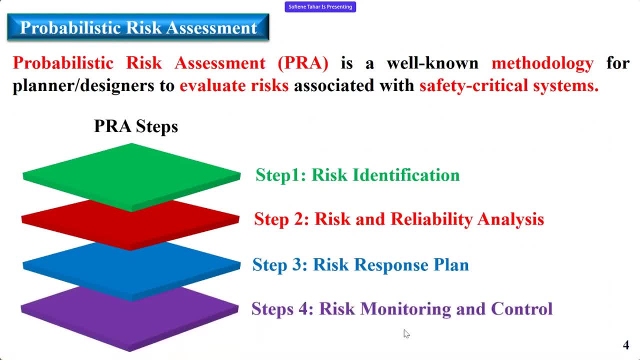 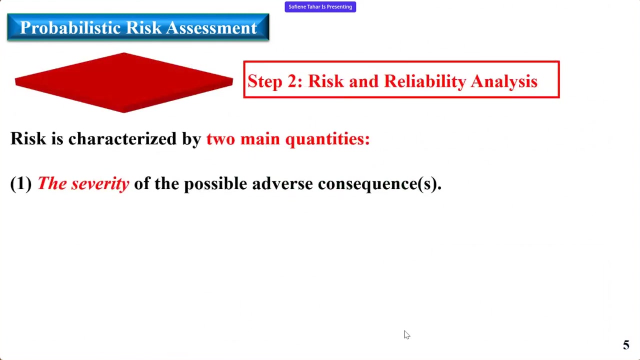 with a risk response plan And, finally, so they have to implement some risk monitoring and control system. We are interested in this work about risk and reliability analysis, So we're not working on identification, nor a response plan, nor monitoring and control. All right Now. the risk and reliability analysis can be characterized by: 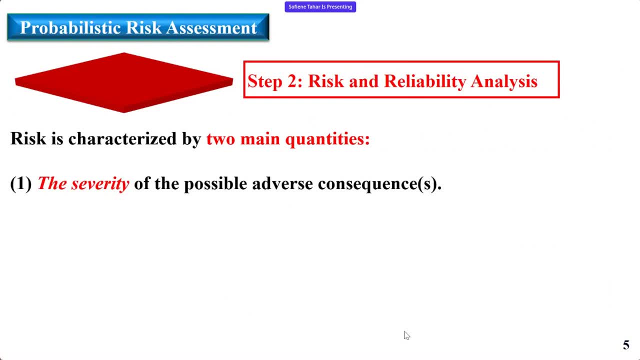 two quantities. The first one is the severity of possible adverse consequences, And the second one is the likelihood of the occurrence of each of these consequences when you know an accident occurs. So this is basically the likelihood of consequences that are usually expressed as 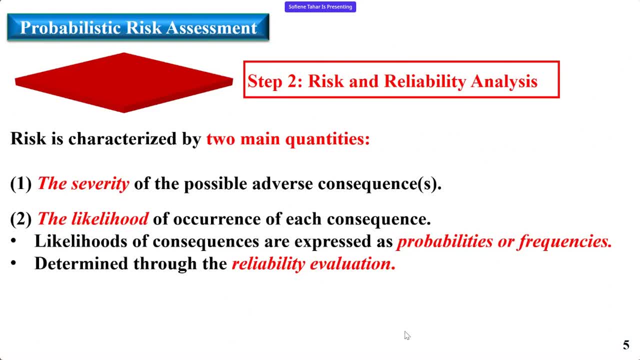 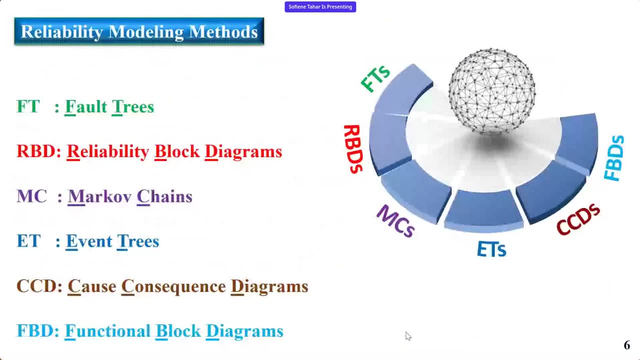 probabilities or frequencies and that are determined through some reliability evaluation techniques. We distinguish here reliability modeling methods as well as reliability analysis methods. So there exists different modeling methods, you know, for reliability, as many of you know, So for 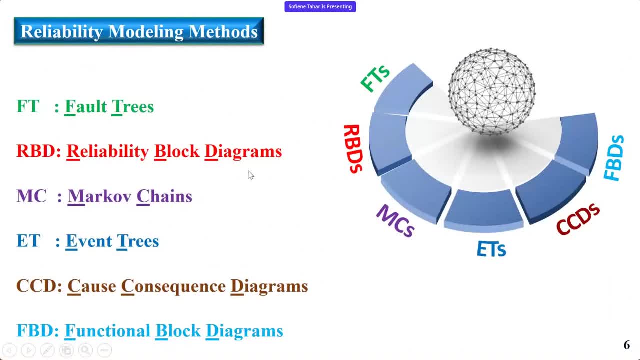 example, fault trees, reliability block diagrams, Markov chains, event trees, cause-consequence diagrams or functional block diagrams, which are basically the main modeling method that I'm going to use in this work. So fault trees, as you know, they model the probabilities of a system. 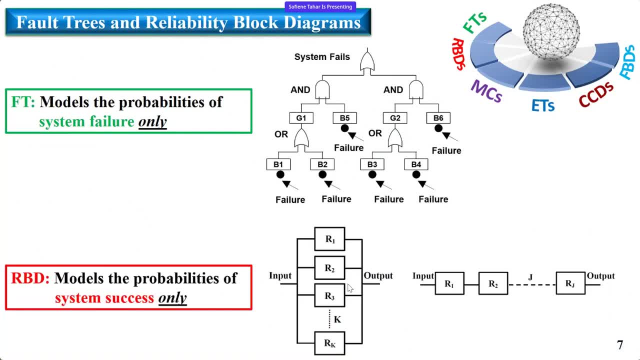 failure only So, while RBDs, or reliability block diagrams, they model the probabilities of system success only. So basically here, so we start with a system and then so we go through different paths and then we actually find you know the failures, while with the RBDs, 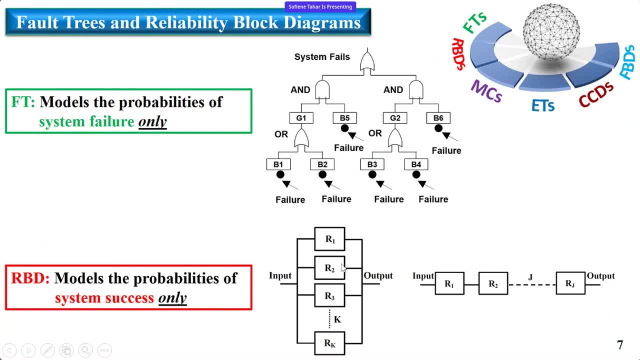 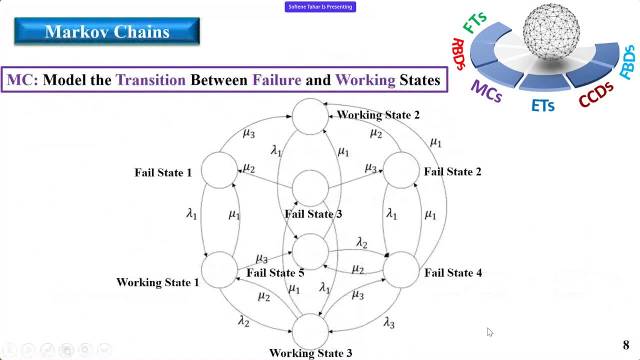 basically. so we have here the block diagrams that are either here in parallel or they are in parallel in series, And then, you know, the success will depend on, for example, each of these to be successful in order to get an output with no failures. Markov chains are also very much known. 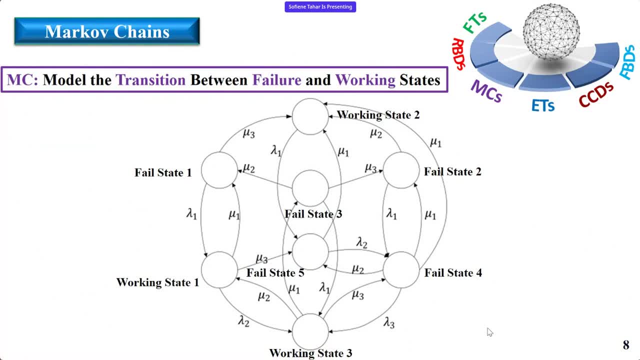 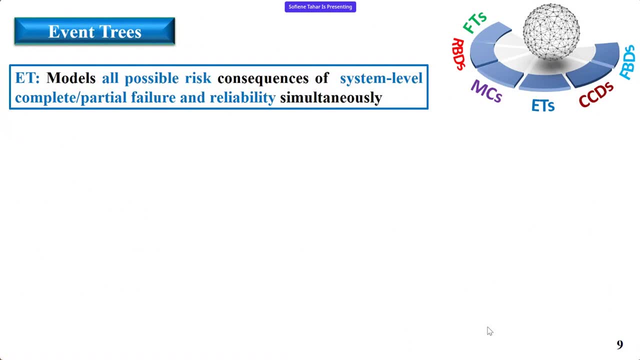 And then they model the transitions between failures and working states, Now event trees, which might be new to you. they model actually all possible risk consequences of system level complete or partial failures, as well as reliability simultaneously. So basically we start here with an initial node And then actually a state could be a success. 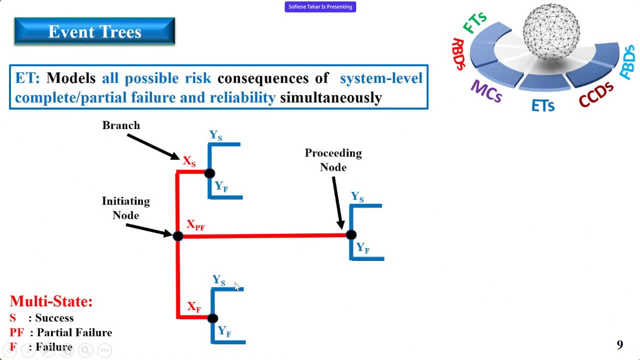 a failure or a partial failure, And then so we can have branches, And then out of one branch so we can have another node, And then so we can continue actually with further nodes and branching, And then each of these, so again, 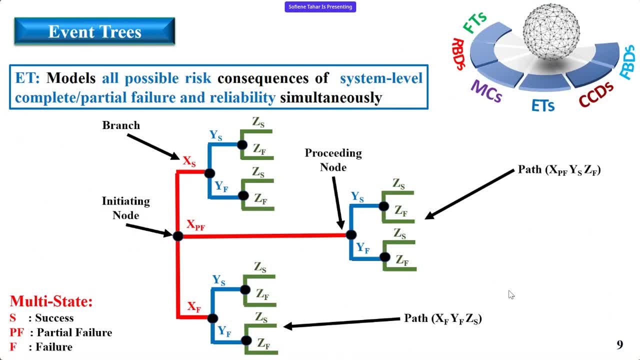 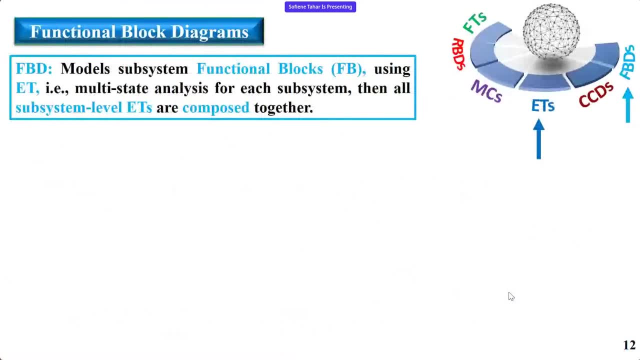 will carry multiple states. that could be a success, a failure or a partial failure. Now, functional block diagrams. they are built on top of event trees And they allow multiple state analysis for each subsystem. Then, at the subsystem level, event trees are composed together. 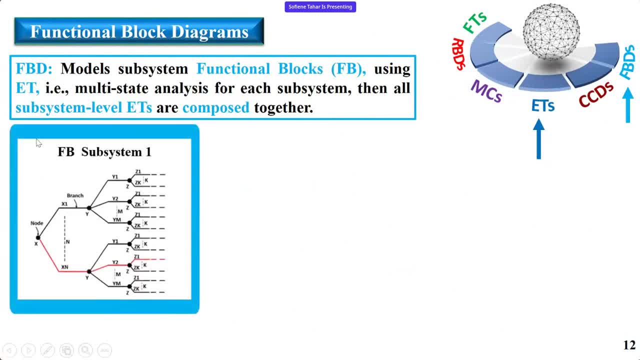 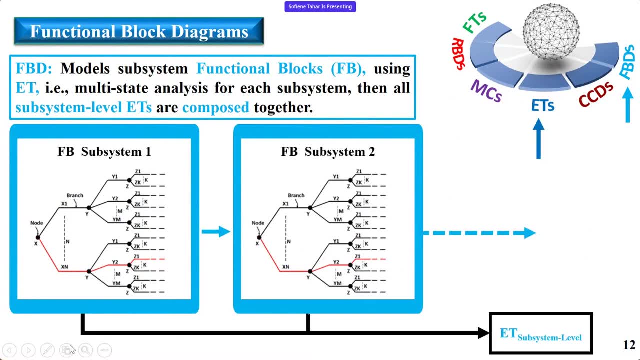 to make the functional block diagram. So, for example, this is the functional block diagram, system number one, And this is system number two, And then together so they compose, if we flatten it, a huge event tree, But it allows us basically. 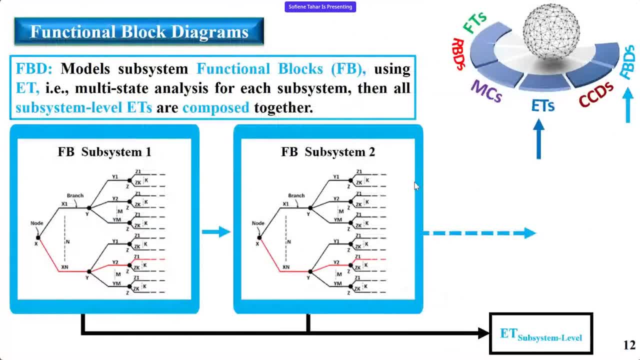 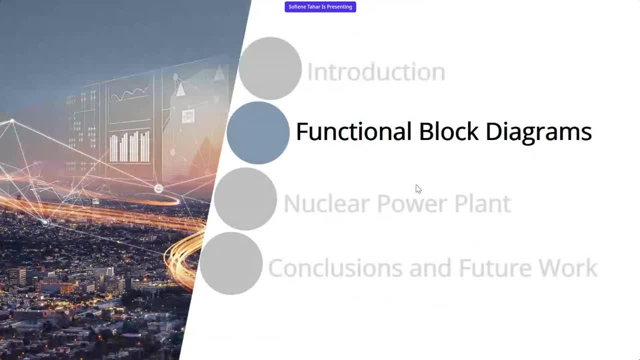 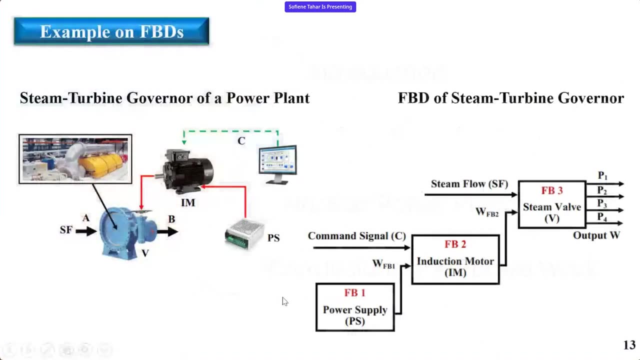 to reason at the block level. That's why they're called functional block diagrams. So let me show you an example of a functional block diagram so that you understand basically the modeling behind it and how it works. So this is an example of a steam turbine. 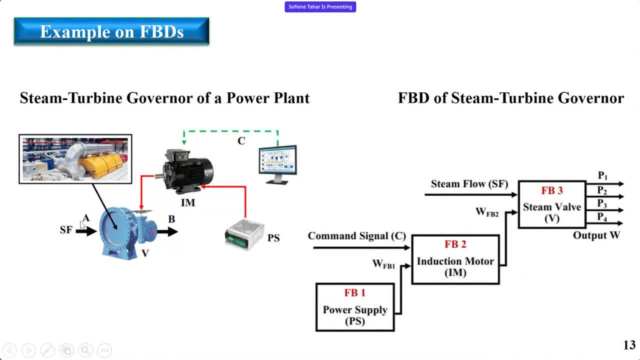 governor of a power plant. So it is composed actually of a power supply that we find here, There is an inductor motor And there is here a steam valve And then through that so we have a steam flow. basically that goes through this with a control here through like a monitor Now, in order for the system to 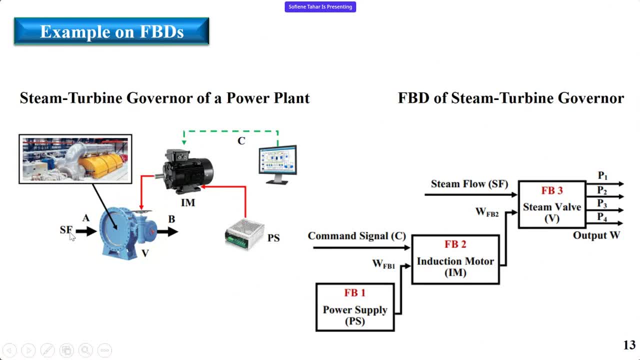 work properly. so we have to make sure that through the flow so we have actually no failures. So if we now model each of these blocks with a functional block diagram, then, for example, here we see the functional block diagram, one of the power supply which is in here And 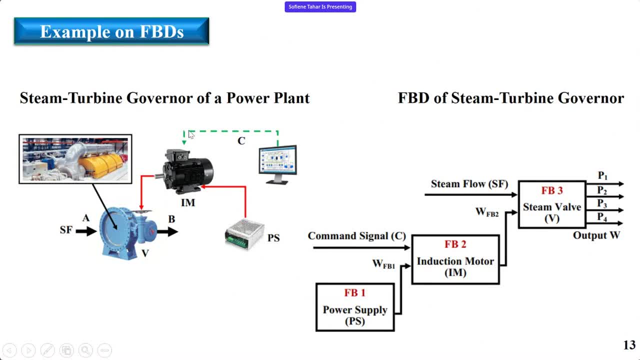 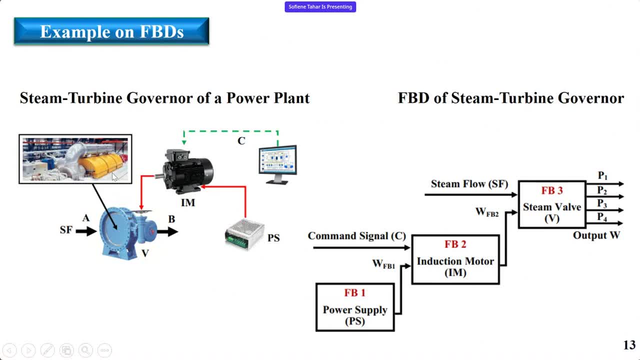 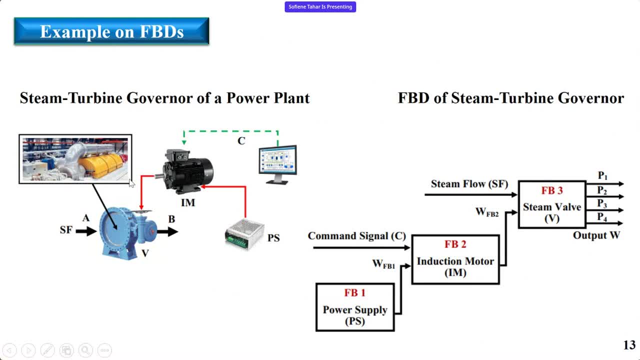 the valve is controlled through the motor- okay, the induction motor, then. clearly, here we can notice that if the computer fails or the power supply fails, then nothing is going to work. or if these two actually are working, but the motor fails for whatever reason, then i cannot control the, the 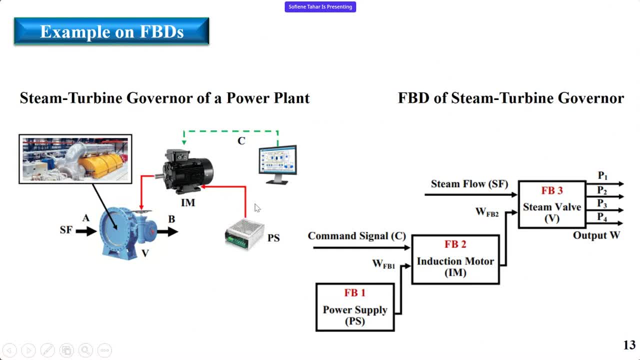 valve right, and that's how we know the dependencies actually are taken care of. and this is all represented through this diagram here, which is the functional block diagram of the whole steam turbine governor, which is composed of subsystems. so we care about the reliability analysis of every. 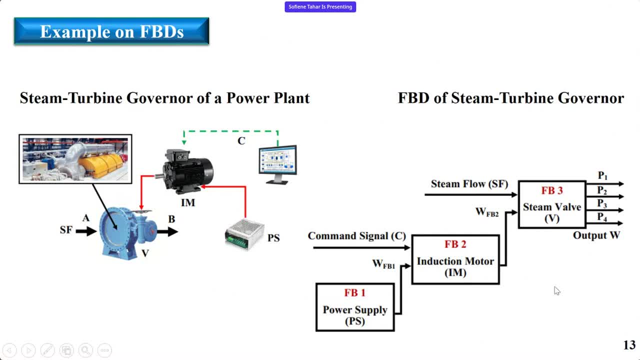 subsystem in order to make sure that the whole system is working properly. now, p1 to p4 are here, like you know, properties that we want to check, and then for each of these properties, in order to be valid, so each of these subsystems has to work properly. all right, now how do we model this? 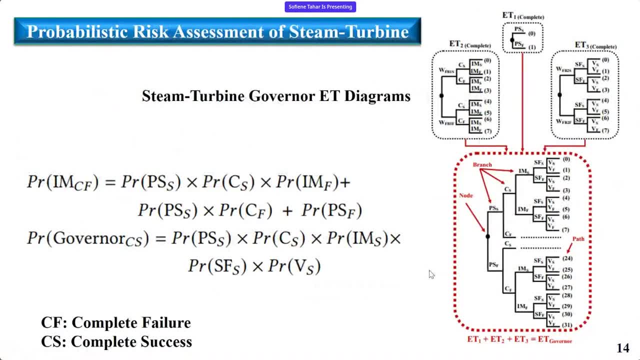 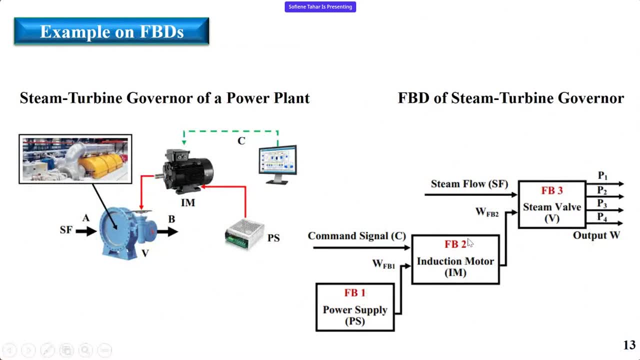 formally. well, it boils down all to probabilities. so i was mentioning earlier that if this one fails, for example the power supply, then if this one fails, and so forth. so any system that you have, any component that you have in any system, you are given a specification and in that specification 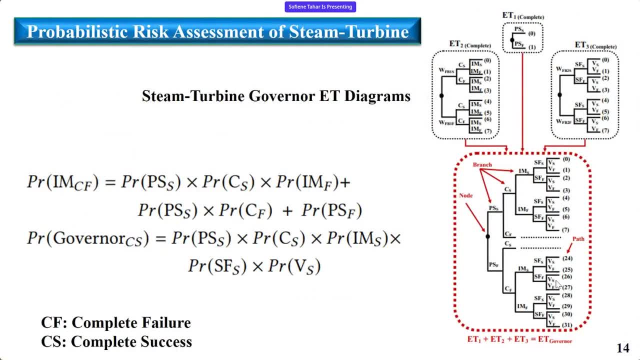 you are told that this is the, that particular component can fail by a probability of, for example, 0.0001 percent, or it's going to fail after you know 10 years, or you know 20 years. so these are probability values that are usually provided and, in order to compute, 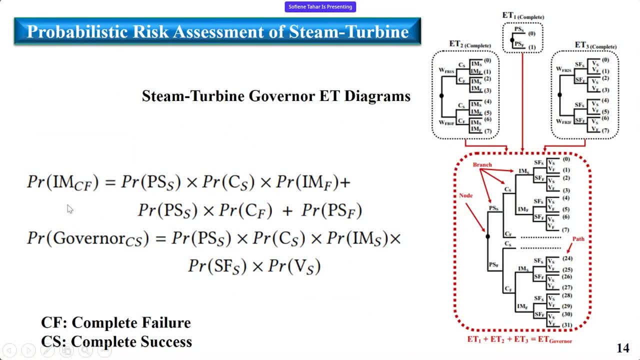 the probability of failure of the induction motor. that is here. then this is depending on the power supply probability. okay, so this is probability of success and then this is probability of complete failure. so, cf, so we have here basically the probability of the power supply working successfully. then this is the control, also successfully. 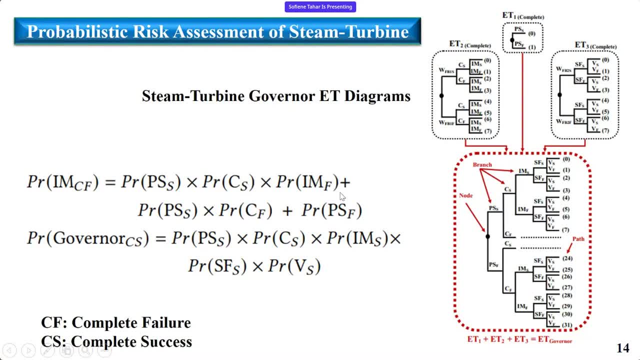 but if we have a failure here of the, of the motor, then you know we can have a failure of the whole system. plus we can add the probabilities of successfully working of the power supply, multiplied by the probability for the failure of the computer, plus the probability of the failure. 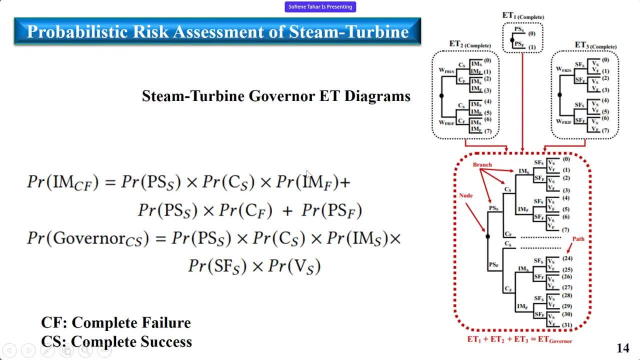 of the power supply and then. so this is all together providing the probability of the complete failure of the induction motor. so similarly, we can reason about the whole system right as being the multiplication of all these probabilities to fail. now as a diagram, so you see them, all them, here described. so this is the first functional block diagram, the second one, the third, 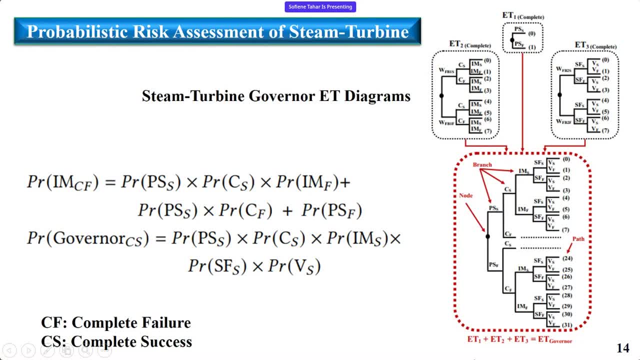 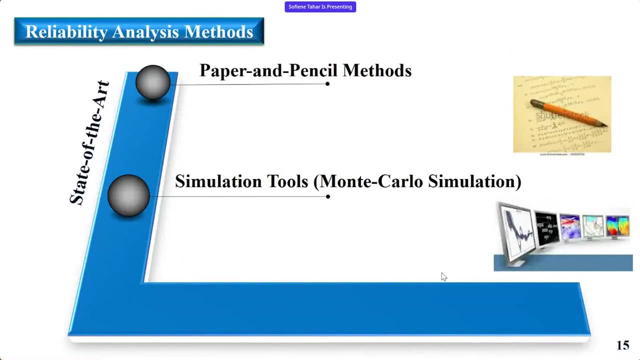 one and then all together. so they make the functional block diagram of this steam turbine governor which, when it is flattened, it's all composed of event trees. all right now, what do people use for the reliability analysis of event trees and, eventually, functional block diagrams? well, paper and pencil methods as well. 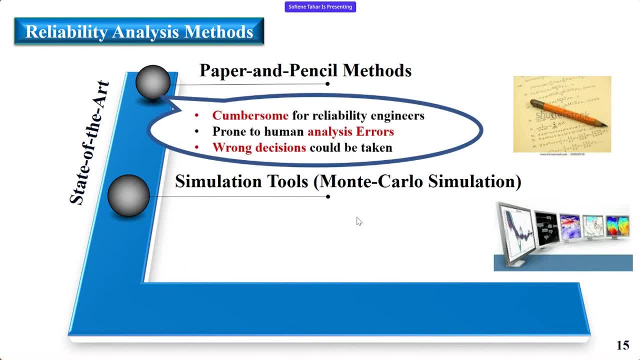 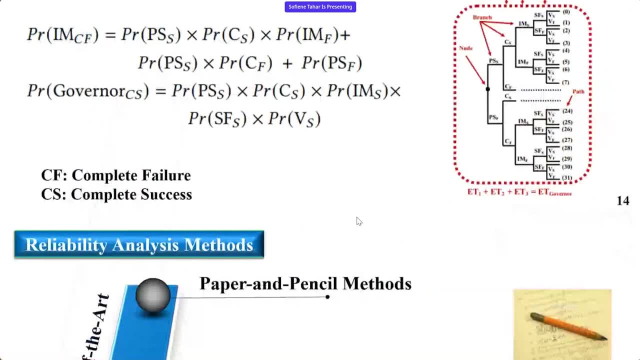 as some simulation tools such as, you know, monte carlo simulation. but we know, all of us, you know that paper and pencil can be very cumbersome, so this is just an example of a very small system. so imagine that we have a system that is very small and we have a system that is. 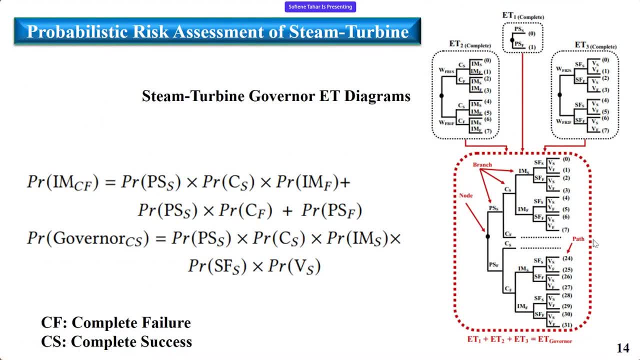 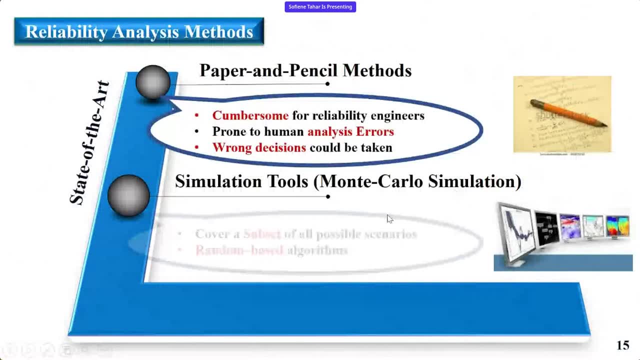 the system has like hundreds of components, it will be very, very hard actually to just draw that. and then you know, compute all the probabilities by hand for the simulation. we know very well that we can only cover a subset of all the possibilities and then so they are very much based on some. 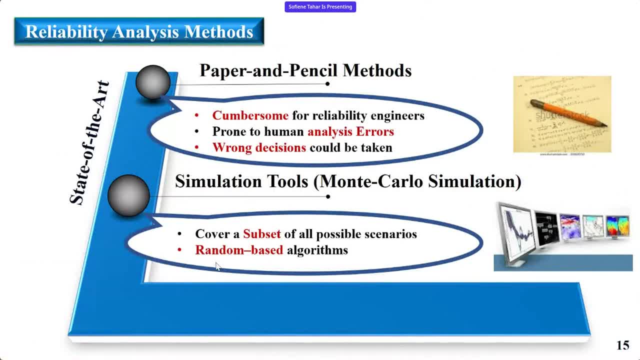 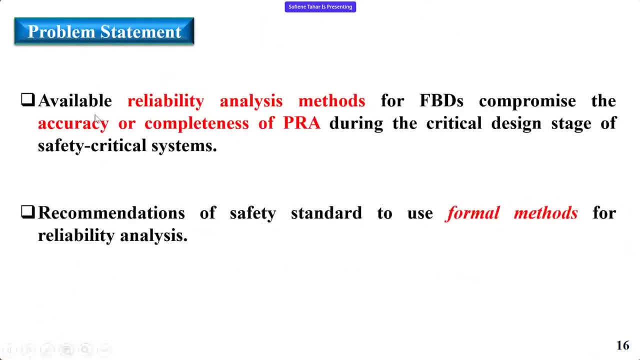 random algorithms which are subject to failures. all right, so what do we want to do in this work? we want to use actually available reliability analysis methods for fbds, and then we want to accurately compute the probability of risk. now, we don't want to use simulation, nor paper and pencil. 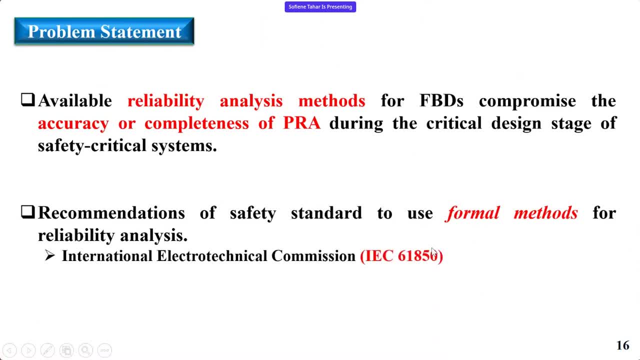 but we want to use formal methods, you know, to conduct that. so now this is recommended by several standards, like the one for electromechanical commission or the european commission or the community for electro technical standardization or the international standardization organization, and this is actually what we are trying to do in this work. in particular, we want to do: 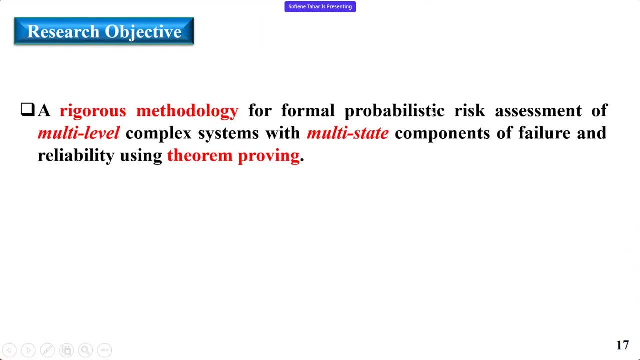 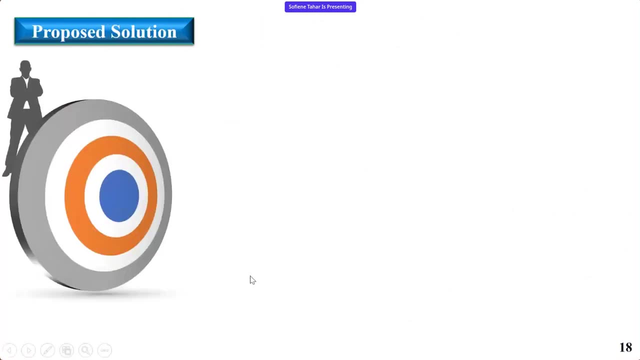 actually the probabilistic risk assessment of multi-level complex systems with multi-state components, using theorem proving, and we want to apply it to a particular system which is a nuclear power plant. all right now, how are we going to do this? so far, because this is the конкретizing and 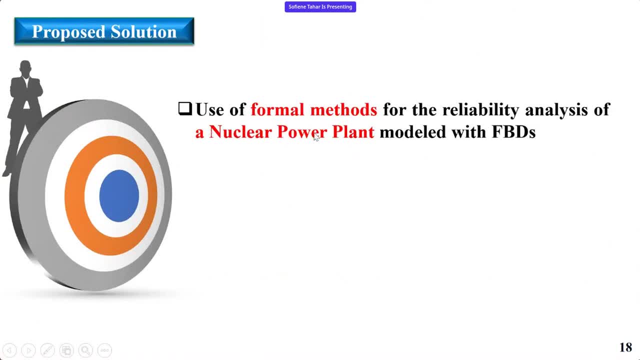 Now, how are we going to do that? So the nuclear power plant is modeled with the functional block diagrams And we use higher-order logic theorem proving, which is capable to reason about multiple-level and multi-state of complex systems. So if we use, for example, model checking or we want to use first-order logic, automated theorem provers, then we don't have these capabilities. 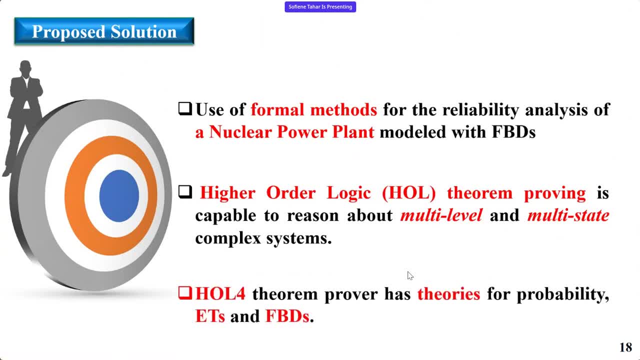 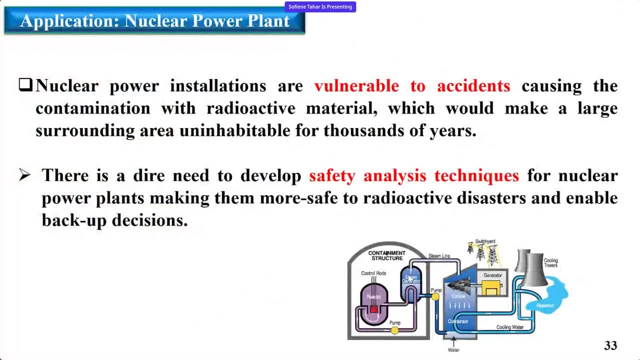 In particular, we use the whole-four theorem prover in order to conduct the probability analysis. Now let me talk quickly about this nuclear power plant that we are considering. So we know very well that nuclear power plant installations are very much vulnerable to accidents, which basically can cause a contamination with radioactive material. 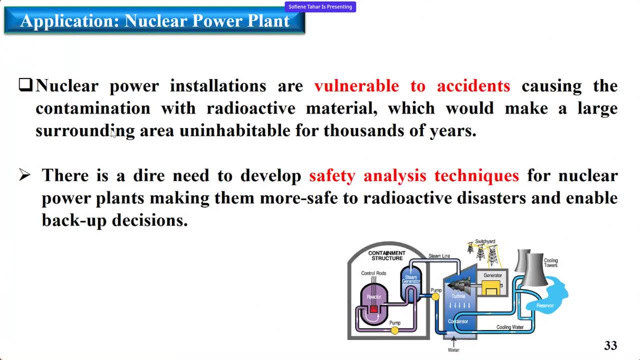 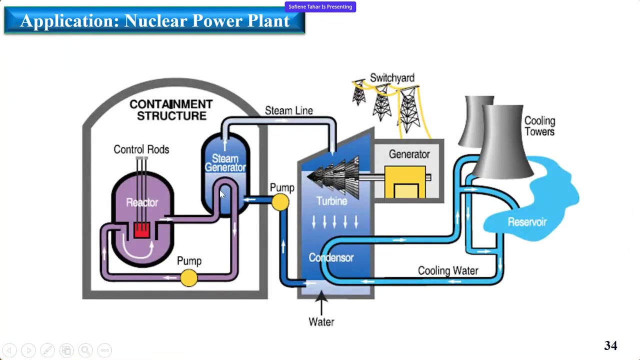 And this would make exceptions- Actually a large damage to the surrounding inhabitants or basically the environment as a whole. So there is a dire need to make sure that these are safe, And then we want to avoid radioactive disasters. Now this is basically a diagram of the structure of the nuclear power plant. 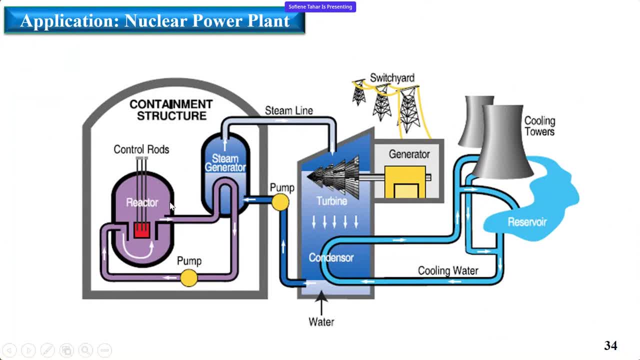 So first we have here a nuclear reactor which heats the Reactor coolant, which can be water or gas After that. so we have the reactor coolant that is passing through a steam generator which heats water and produces steam flow that goes through here. 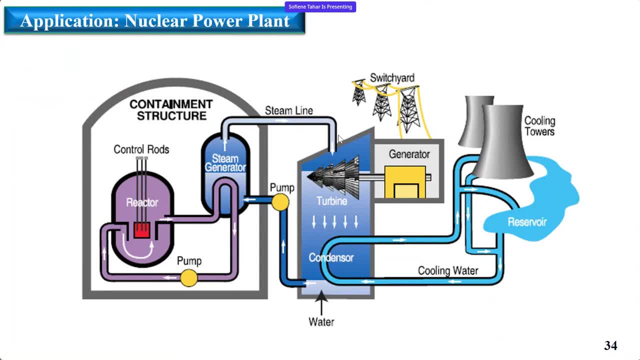 And then after that. so we have some pressurized steam flow that goes through the steam turbine, which then starts to produce power, And then the remaining vapors actually is condensed through the condenser. So the condenser basically is used to exchange heat through a secondary side. 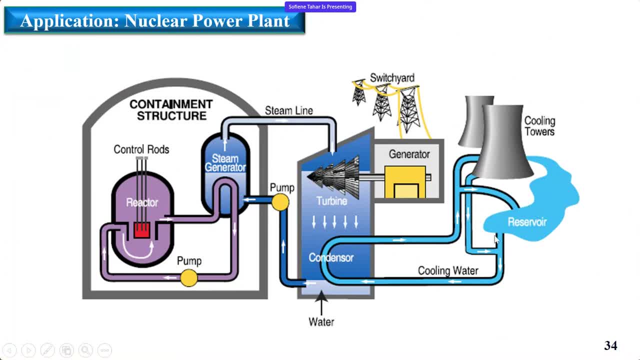 For instance, we can have, like you know, a river or lake, OK, so that you know the this condensed water you know can be go through here and then so it's cooled, But you know we can reverse the direction and then we have the cooling water coming back, so that you know, again we can use it. 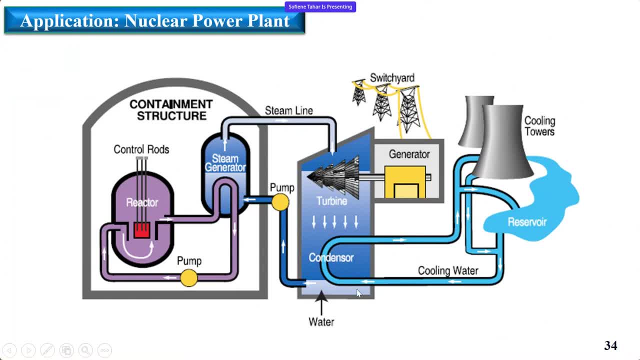 For the steam generator and the cycle you know will be repeated. All right, Now we see here that you know this reactor is composed of several parts and we are interested in particular, for you know this boiling water. boiling water, you know. reactor: 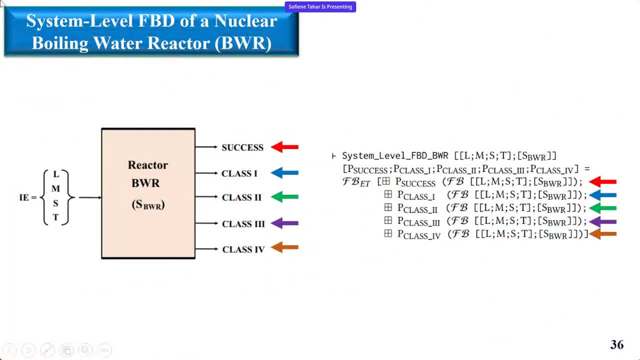 And then so we have here several basically classes that we are considering, And then so we have here several basically classes that we are considering. So we are starting here with some initial events, And these initial events basically could be a large loss of coolant accident or a medium loss of coolant accident. 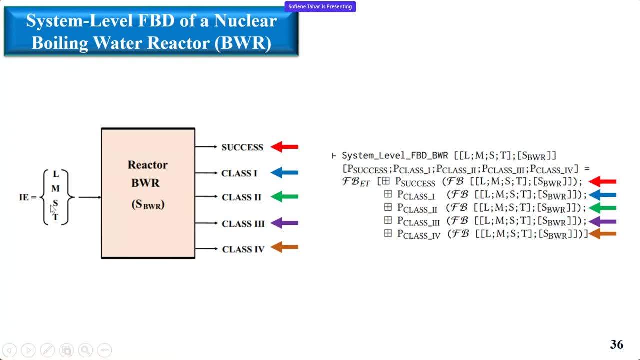 Or it could be basically a small. so here S so a small loss of coolant accident, Or it could be just a transient accident. Now we identify different. We identify different classes of accidents, right, which we are here considering them one by one. 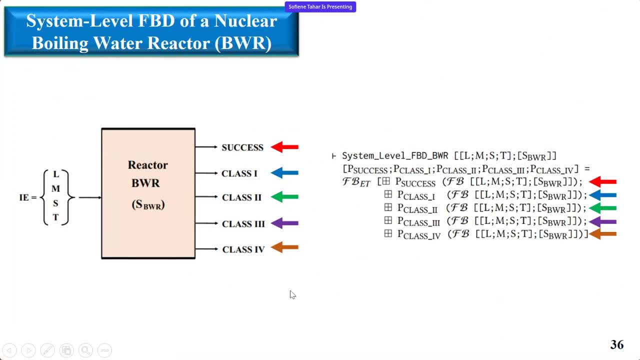 So I'm going to talk about them. you know about each of these later on Now in high-order logic. so I have here a predicate, basically that is describing the functional block diagram, And then so it considers the different classes of accidents. you know that I'm here basically considering 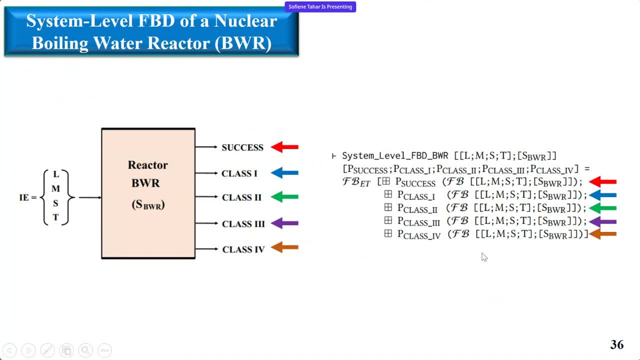 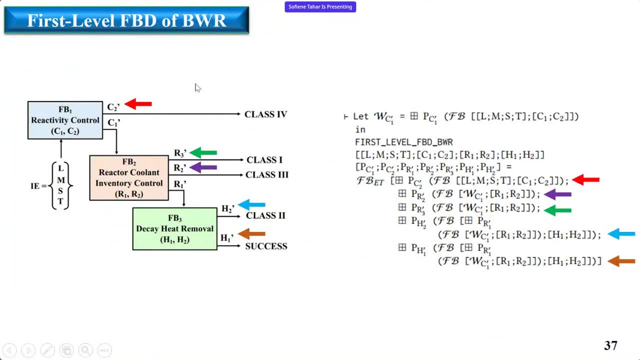 And then so for each of them. So I want to make sure that they are successful. All right, Now again. so this is the functional block diagram representing my reactor. So we have here the functional block diagram representing the activity control, And then the next one is the reactor coolant, as well as the inventory control. 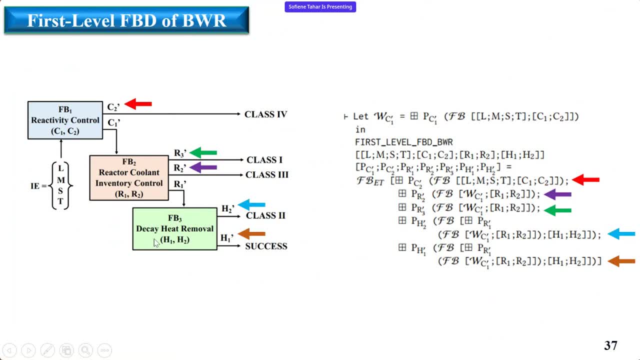 And the last one is for the decay heat removal. So again, each of these is representative, Each of these is represented as a predicate, and I use this particular operator which takes basically the output of an event tree model and then a partitioning of events and then after that, so I can have reasoning about the reliability of these events. 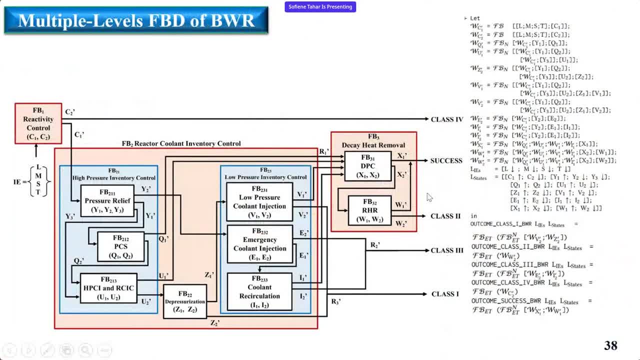 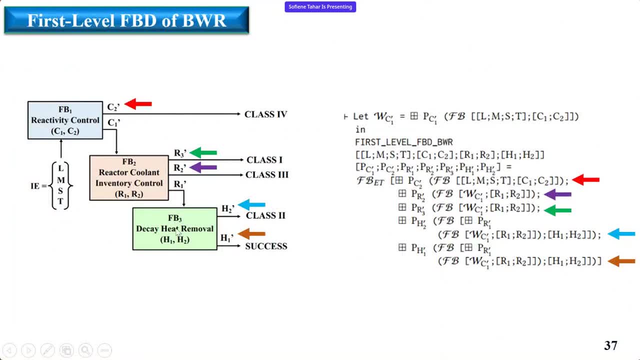 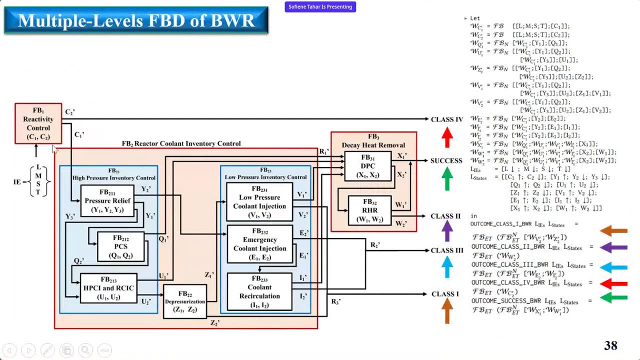 All right. Now I think this one, which is basically the larger view, Yeah, So each of these blocks now contains sub-blocks. So the first one So is we have here the reactivity control. After that we have the reactor coolant and the inventory control. 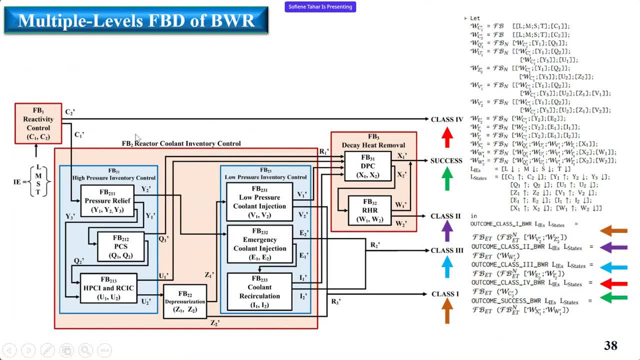 And then, finally, we have the decay heat removal. So if you look at this functional block diagram number two, it's composed of two sub-blocks- One is for high-pressure inventory control and another one for the low-pressure inventory control- And inside each of these blocks we have again sub-blocks. 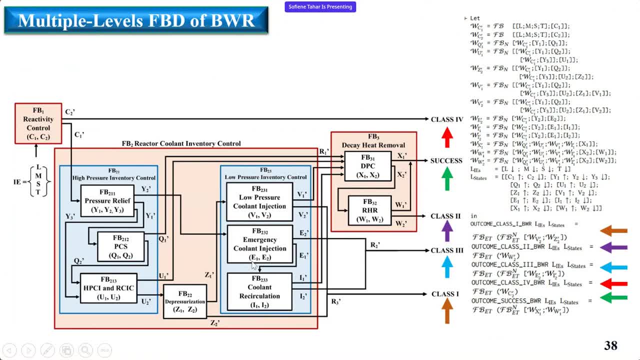 So one is for pressure relief and then so we have, you know, other ones. So, for example, here for coolant recirculation and so forth. Now, the beauty of functional block diagrams, as I mentioned earlier, is that we can have actually a hierarchy of blocks and then sub-blocks, and then sub-sub-sub-blocks. 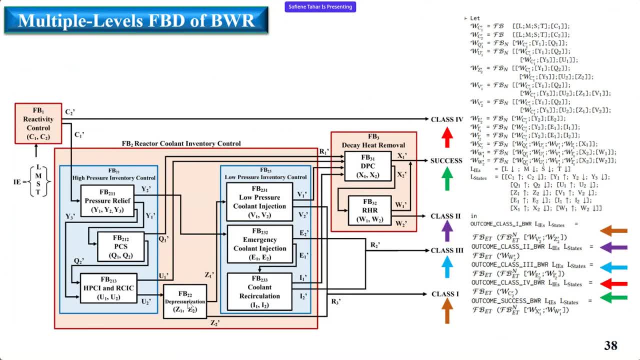 So we have multiple levels And then in every level so we can have multiple states. So it's not just failure and success, but we can have failure success or complete success, or complete failure, or partial success and partial failure. 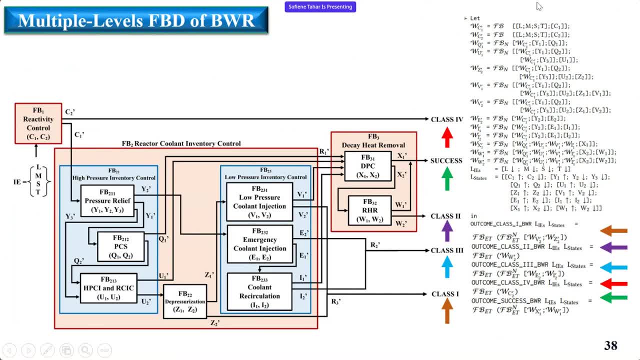 And then this is all now combined together in one large predicate. This is the one you see on the left side. Probably is too small, you know to see, but you know this is how this is composed in high-auto logic. 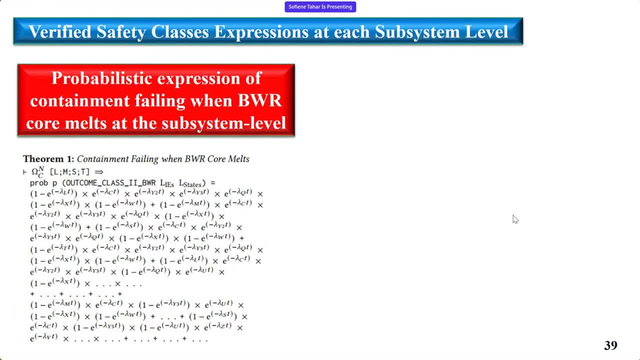 All right, Now we have proofs. We have proofs of the number of theorems. So, for example, this theorem number one is about the containment failing when the boiling reactor core melts. Then this is described as Your talk in as much as possible, because it's kind of over. 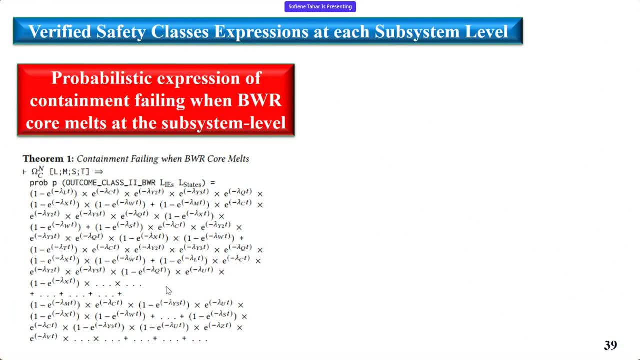 Sorry about this. Okay, Can I continue? Yeah, sure, Okay, So I'm almost done So here. basically, if we see about this theorem, so it's a multiplication of different probabilities, And then this is taken into consideration. 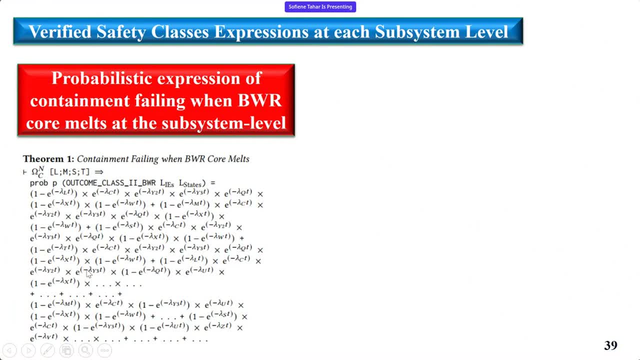 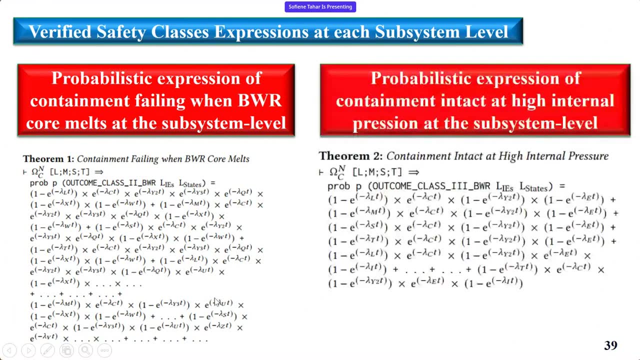 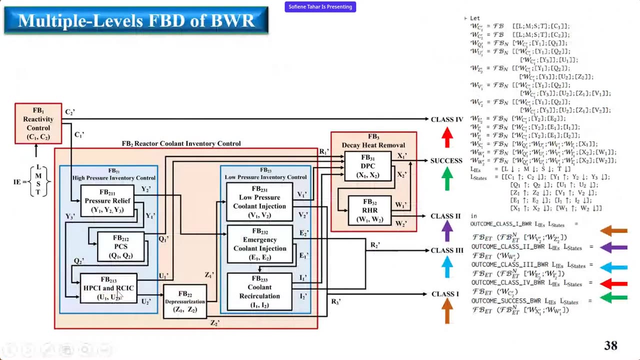 So each of these, exponential to the power of minus, you know delta here and so forth. So each of these is representing one of these blocks, right? So this is the probability of failure of each of these subblocks. That is probability. 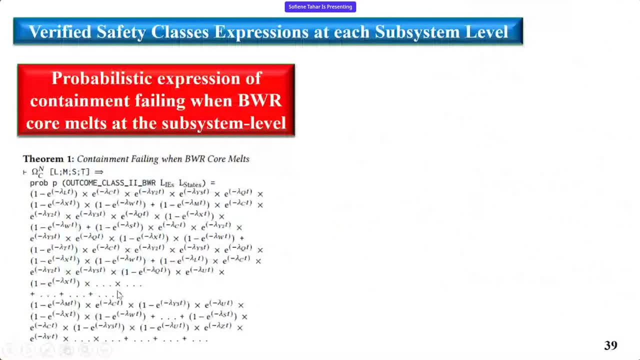 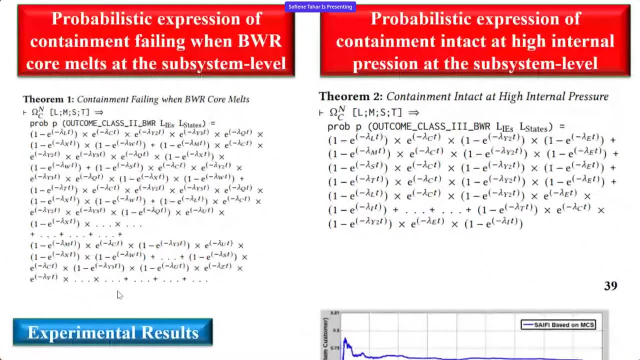 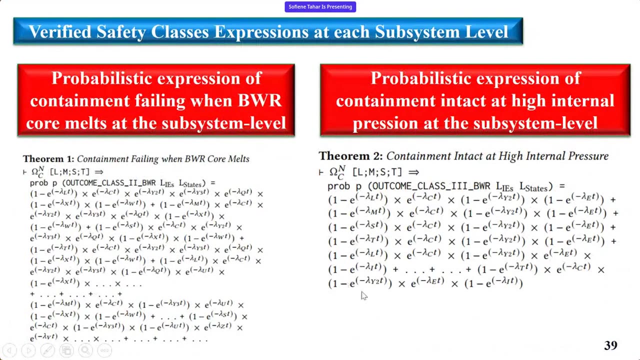 And then this is divided by the vendors, basically from where we buy them or they are basically making them. So this is another theorem, basically for the containment of intact at high internal pressure, And again it is a multiplication of all these, you know, failure probabilities. 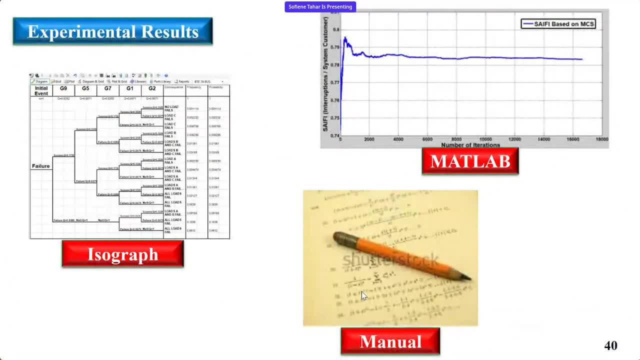 All right, Now we wanted to do some experimental analysis And numerically we want to compare the results that we obtained through high-auto logic. Well, basically the whole four theorem prover with a number of tools. So one is iso graph. 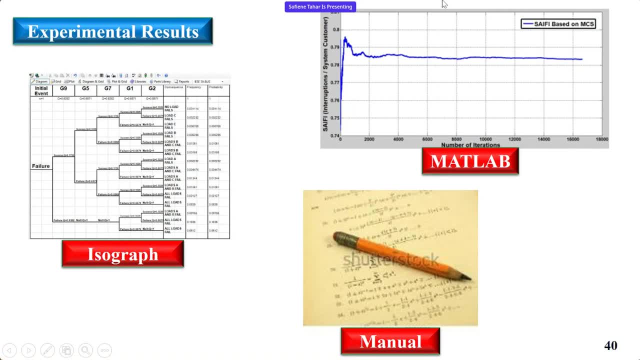 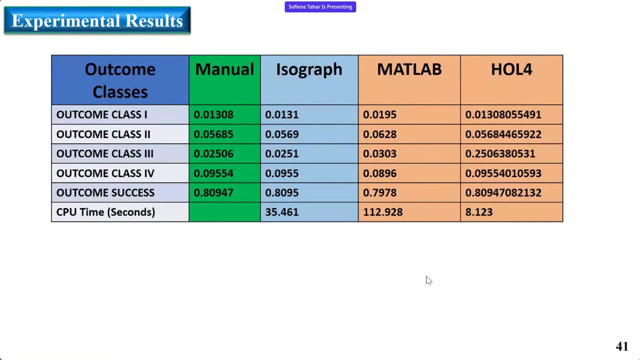 And this is a tool for event trees, It's a commercial tool- MATLAB, and then paper and pencil. So the paper and pencil analysis actually was conducted by a work prior to us And that was the first work. you know that from where we got inspired. 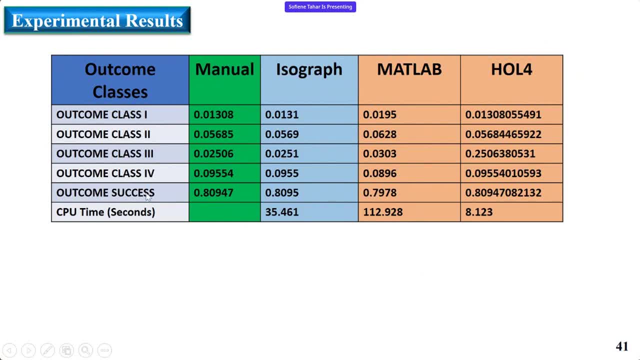 And we have here in this table the different outcome classes. And then there is the, basically the time for their computations using the manual. Sorry, not the time. These are the probabilities of failure and success. So for the manual approach using iso, graph, MATLAB and all four: 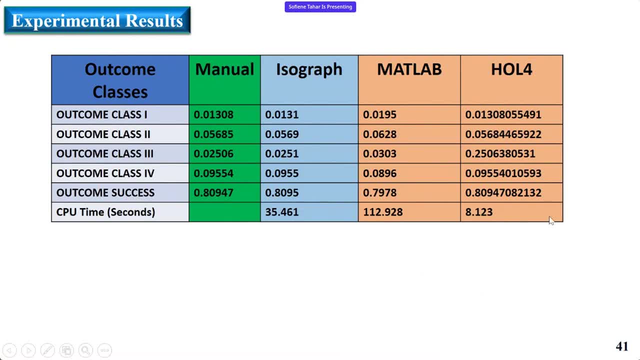 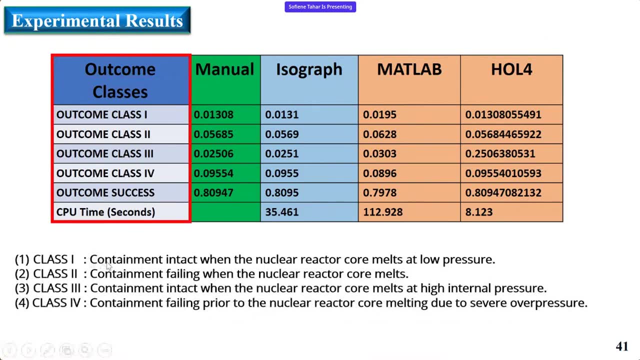 Then the last row here is about the CPU time, where we are doing it on the same computer. So the class number one is basically to check if the containment is intact When the Nuclear reactor core melts at low pressure. The class number two is when the containment fails when the nuclear reactor core melts. 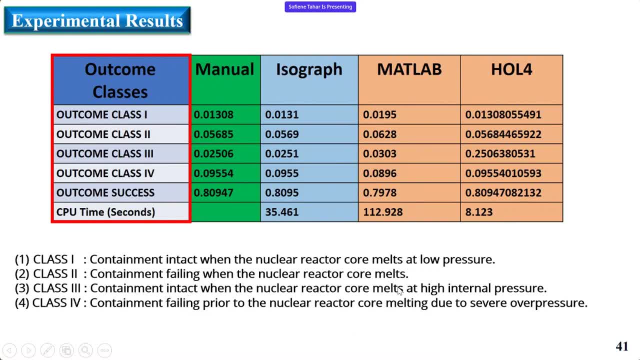 Number three: the containment is intact when the nuclear reactor core melts at high internal pressure. And finally, the last one, the class number four is when the containment fails prior to the nuclear reactor core melting due to some severe overpressure. So these are different scenarios of accidents. 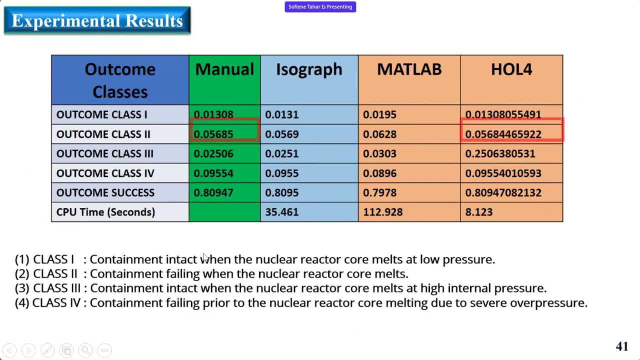 So we consider all Of them with their probabilities And then we notice here, for example, if we compare the manual approach to high logics, we see that we have a better precision here. So we go actually so many numbers you know, after, after the dot. 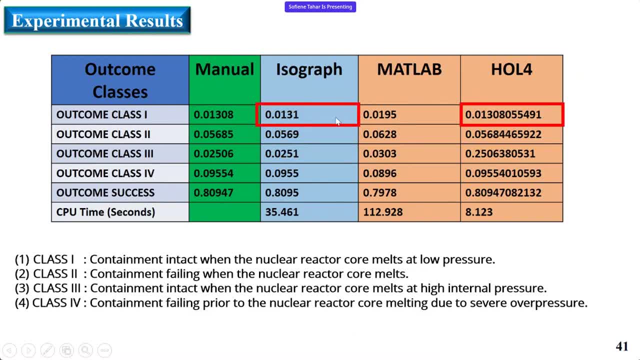 If we compare to iso graph again, so we notice that we are not doing any around in here, but we really have some exact values. So also, if we compare to MATLAB, we see that MATLAB is very far From these value. So basically, if you rely on MATLAB, so you will get the probability of 0.019 instead of 0.013, as you would do it analytically or with you know a specialized tool.